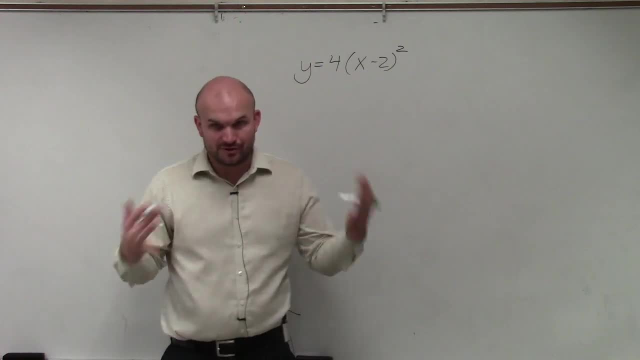 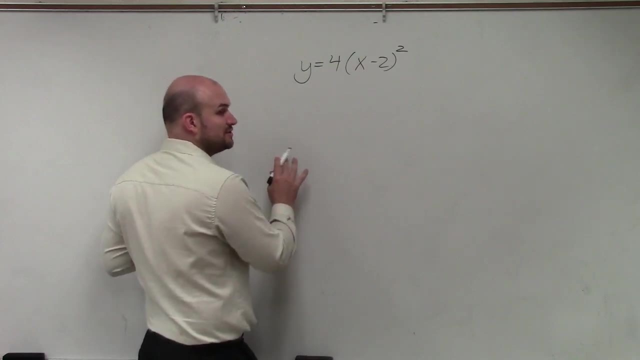 was not a part of it. However, since nobody asked me to do one through six, I do want to go through graphing and make sure. at the same point. However, for all the answers- one through eight- the first two things you guys want to do is identify the vertex and the axis symmetry, So that work is. 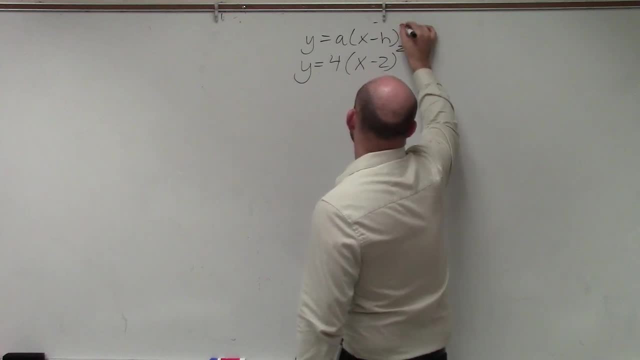 exactly the same And all you guys need to understand for identifying the vertex and the axis symmetry is: go back to your notes. If you guys remember, I provided you with the vertex form of a quadratic And remember the vertex form of the quadratic told us what the vertex was. 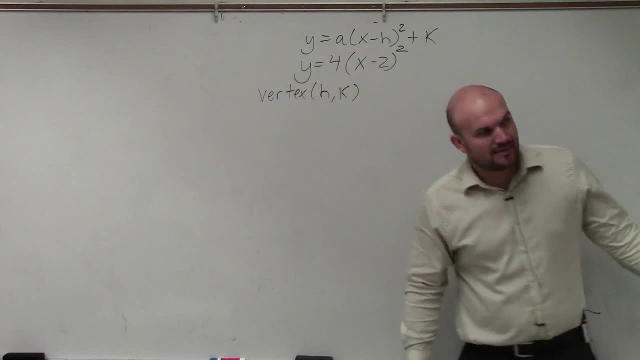 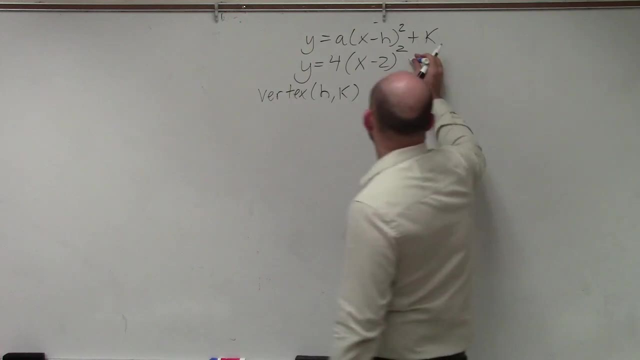 h comma k. So when I'm looking at my problem to find the vertex, all I got to do is identify what is h and what is k. Well, you guys can see I'm not adding or subtracting the number, So we can. 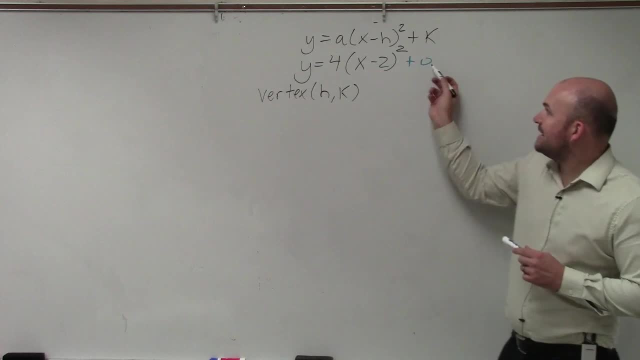 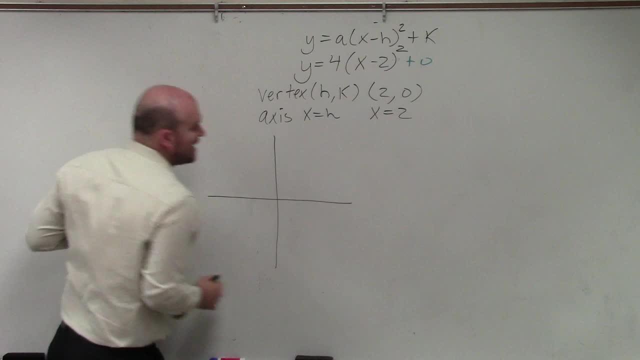 going to do the same thing. So I'm going to do the same thing. So I'm going to do the. So, when you're graphing, the best thing to do is plot your vertex and write in your axis symmetry. So 1, 2, make a nice point. 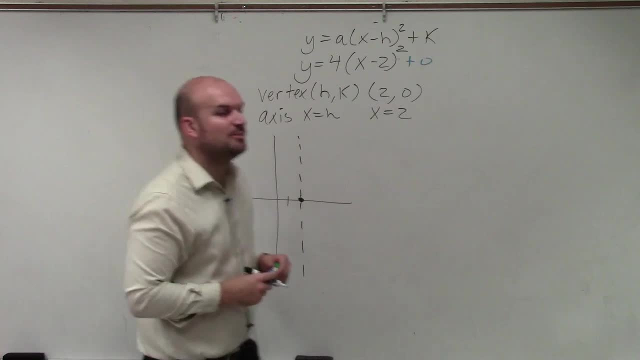 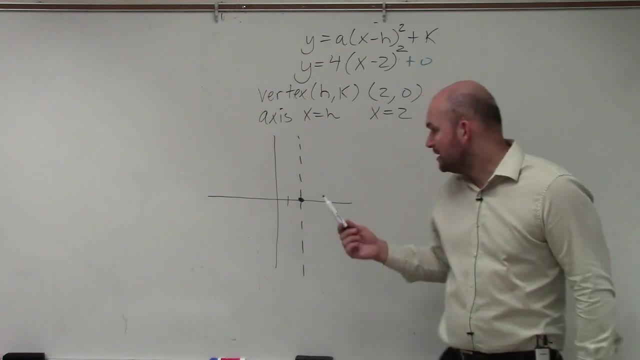 Axis symmetry is the point that the graph is symmetrical about. So if you're having trouble graphing it, the best thing to do, as I mentioned, for absolute value, is just to choose two points to the left or to the right of the axis symmetry. plot them. 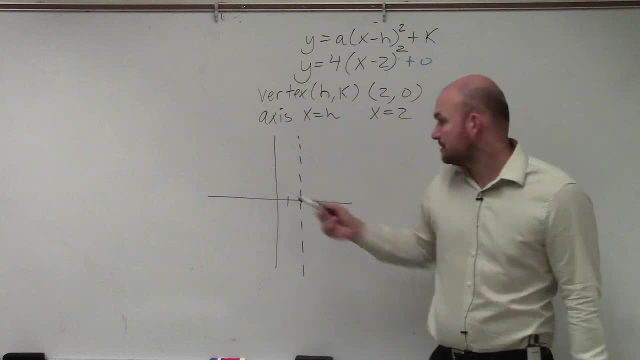 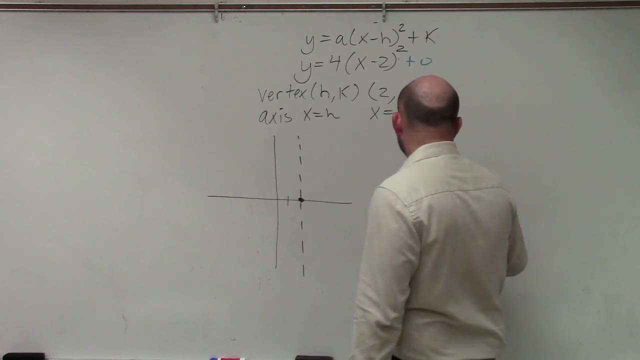 and then you can go ahead and reflect them: Yes, No, OK, However, you guys can go ahead and do that. There's not a problem with that, But I wanted you- I provided you guys with. my points are a little bit off. 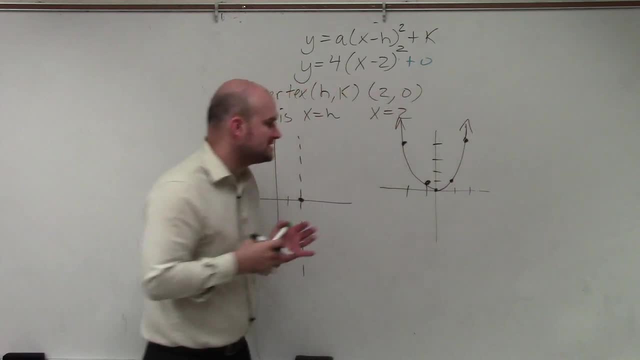 But I provided you guys with the parent graph for a reason: Because I wanted you guys to understand that the parent graph is over 1, up 1, over 2, up 4.. That's for the graph. So what about this first one? 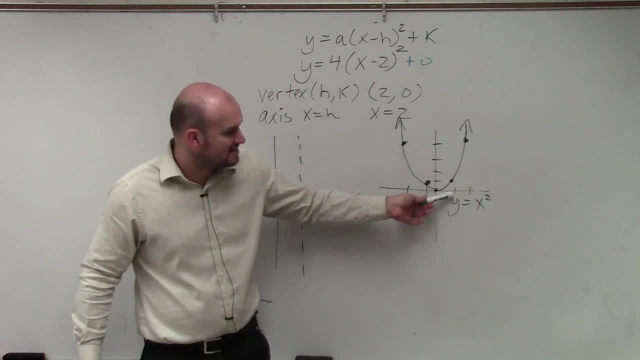 It's going to be 2 over 2.. It's been 2 over 2.. 2 over 2 plus 1.. Two squared. Let's do that again, OK. So 1 over 2 plus 1. Over 2 plus 1.. 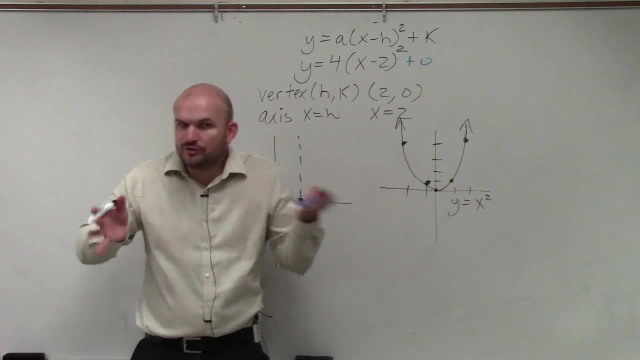 One squared. So now that we're done with the previous one, how about we do that again? If it didn't fit in, how about it fit in here? OK, So what happens? What happens when my x-axis is 2 over 2,? 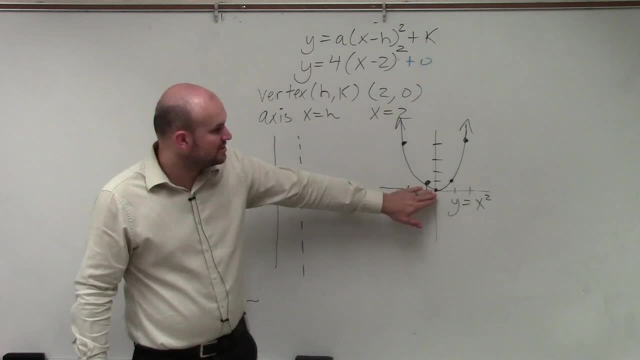 how about I flip it? I flip the y-axis, and that's the same thing. So I flip the x-axis, I flip the y-axis, I flip the y-axis. There's no better way to do it. The problem is if it fits in it's. 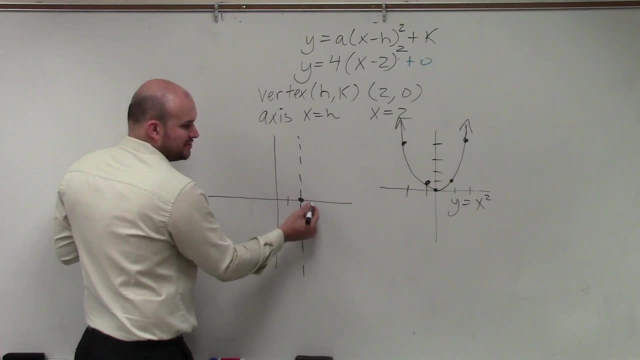 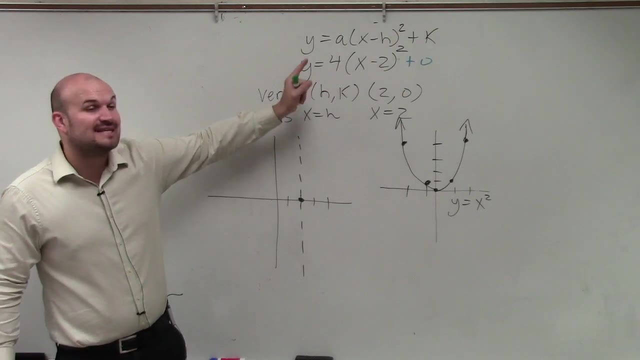 takes being at 0, 0,. I've now shifted over to 2, 0.. Then you just redraw the graph unless you have an a. So my a, if you guys remember, since absolute value of a is larger than 1, that horizontally. 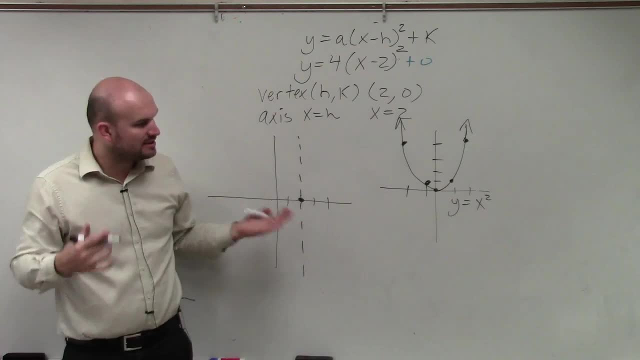 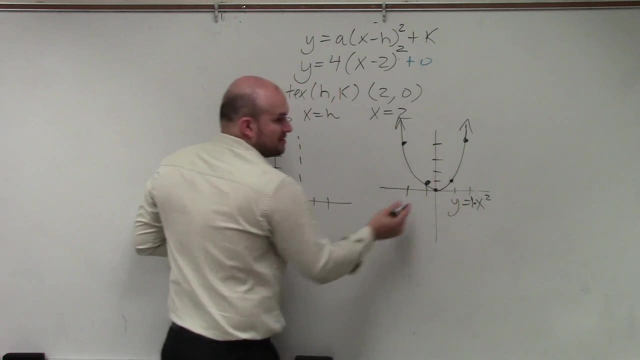 compresses your graph. Well, how does it horizontally compress my graph? If you guys can see here, my a is 1.. So really, when I plug in 1 for x and I square it, I just multiply it by 1, which is the same thing. 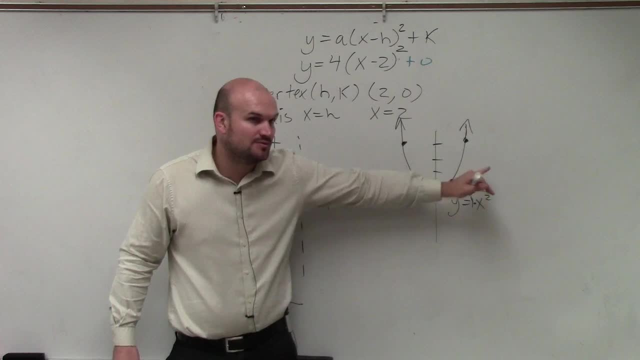 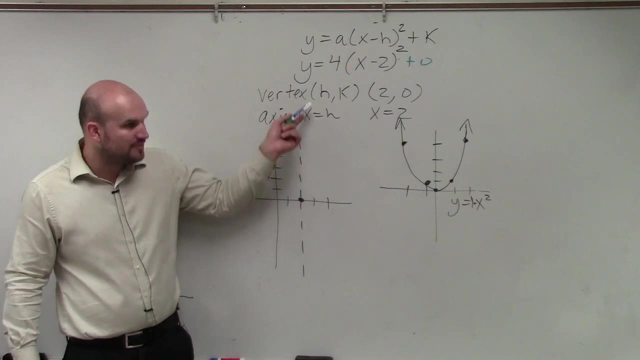 But now that I have 4,, whatever I plug in for x, and once I square it, I have to multiply that by 4.. So, basically, I'm going over 1.. Instead of going up 1,, I'm now going to go up 4.. 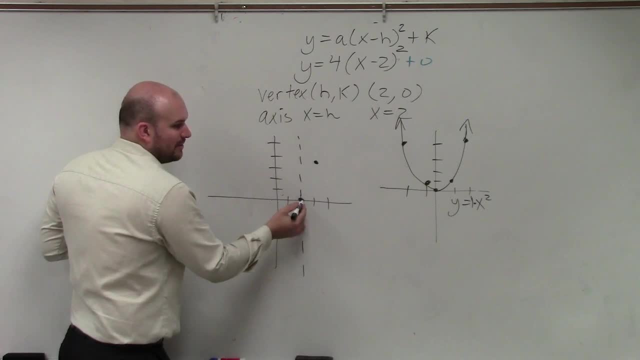 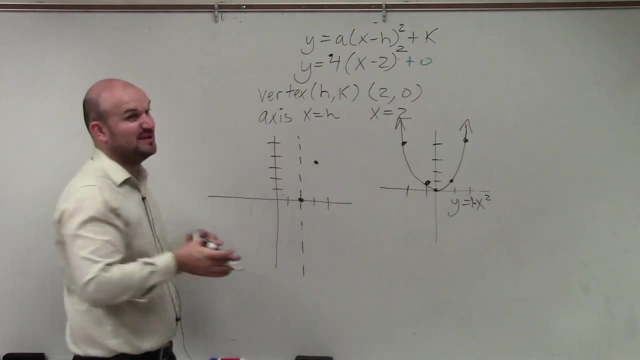 1, 2, 3, 4.. Instead of going over 2, up 4,, I would go over 2, up 16.. So it would be really really high points Now here, Since I know this points to the right. 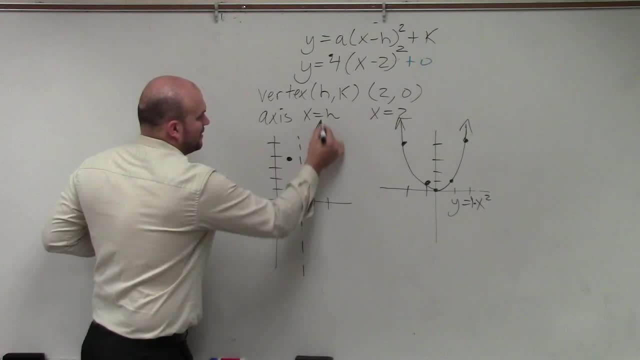 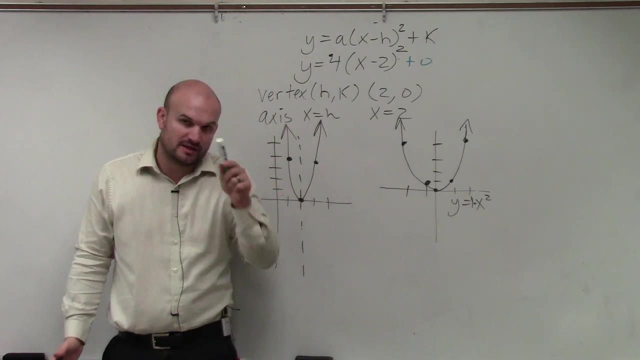 I can use the axis symmetry to reflect it, And I'm just going to use three points here, because I don't have a graph that's big enough. So if you were to graph this problem, you didn't have to do that, But that's what it would look like. 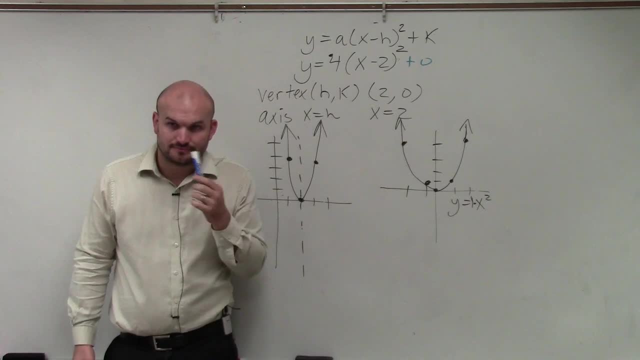 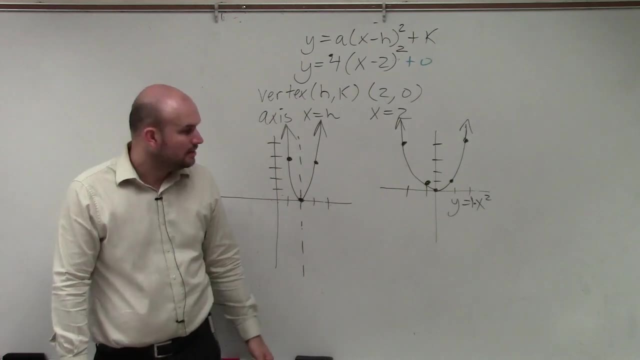 Yes, So basically you just multiply your y according to y By 4.. Yeah, Yeah, basically what you would get when you plug it in, Unless you're going to plug it into the whole problem. Yeah, you basically plug whatever you plug in. 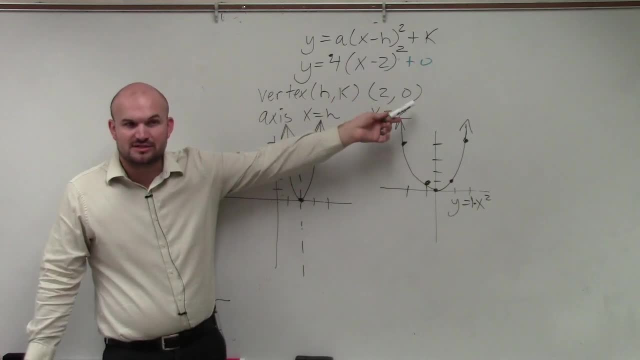 for x, multiply that by 4.. And then, if you had a k, though, you'd have to add or subtract as well, So you have to kind of take in and out. Basically, the best thing, though, is find the vertex which is easy. 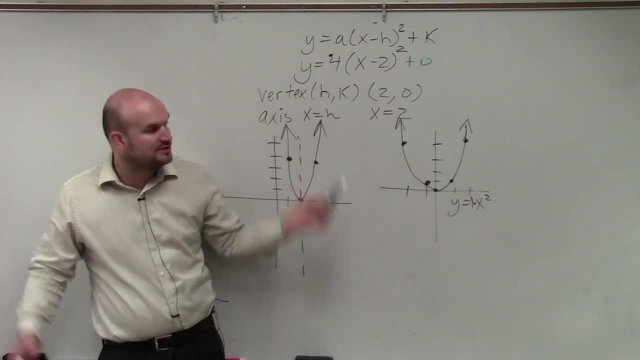 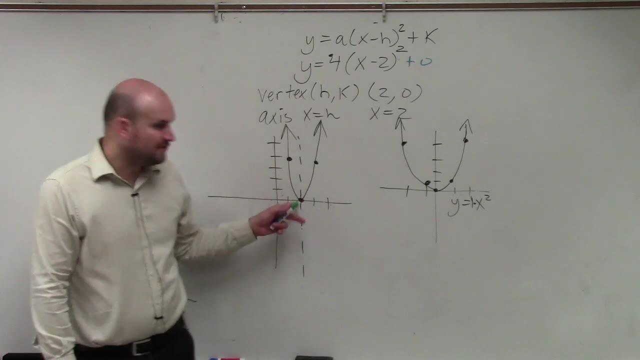 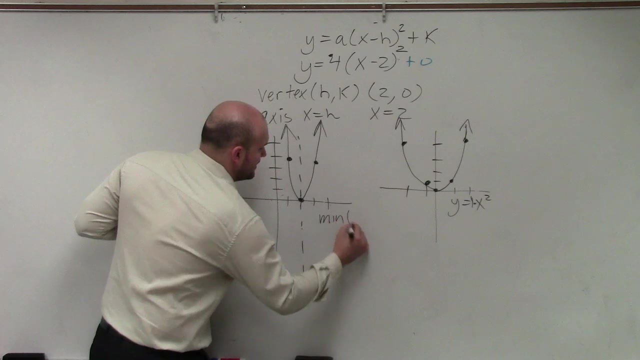 And then you can plug in points to utilize that. So now they're asking for the max and min domain and range, right, Yep? So this vertex: is that a maximum or a minimum point? Minimum point: So you'd say the min is at 2 comma 0.. 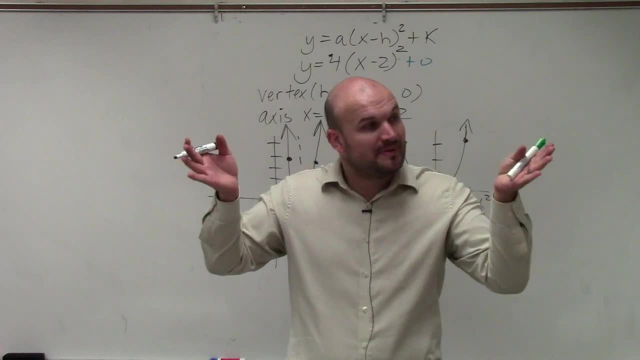 So your vertex is always going to be your maximum, Minimum point, Minimum point, Minimum point, Minimum. But if the graph opens up, it's a minimum point, If the graph opens down, it's a maximum point. Now we need to talk about domain and range, which I'm just 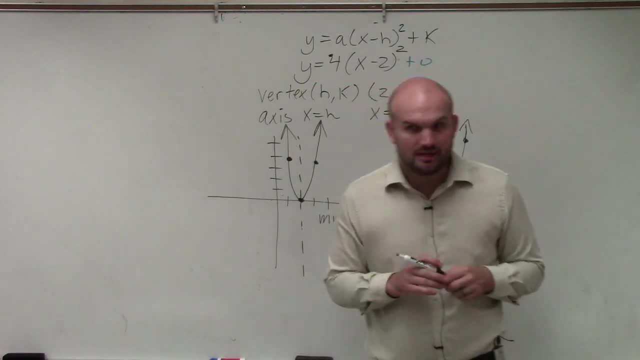 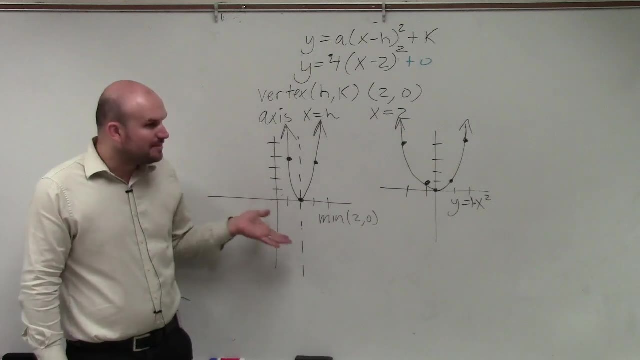 going to introduce to you. We will get into this in much more detail later. So if you're kind of having some confusions, don't worry. I didn't really mean actually to have you guys do. domain and range. The domain and range is the set of all x values. 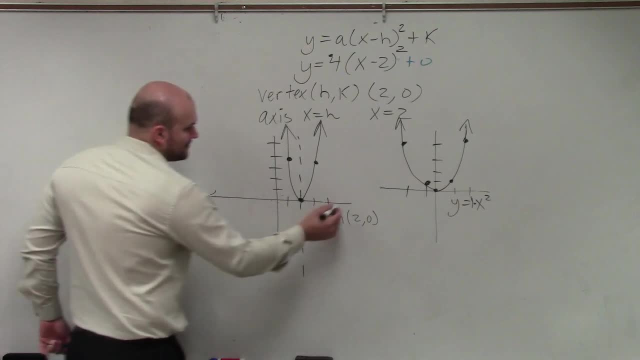 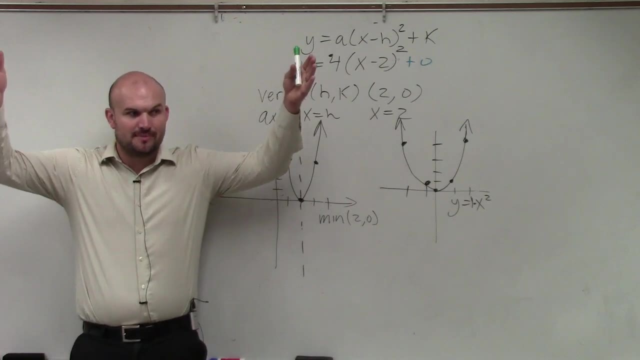 that make up the graph, Meaning how wide do I need to expand this x-axis? Because is this graph going to keep on expanding, go to the left, to the right, As it goes up Right. So the graph is going to go infinitely left and infinitely.